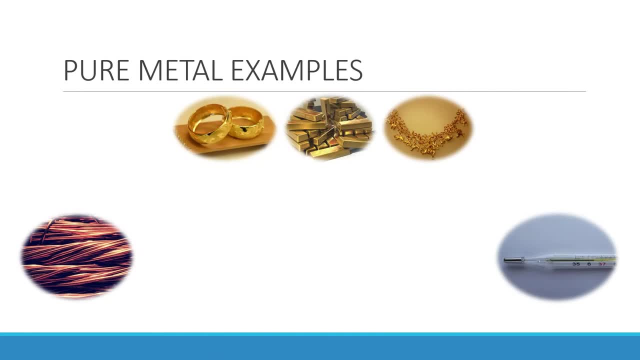 examples: Gold is a well-known women accessories. that some of these jewelries are made from high-quality metal. Gold is a well-known women accessories. that some of these jewelries are made from 100% pure gold atom. Well, I'm sure you have heard of 24 karat gold, which means these types. 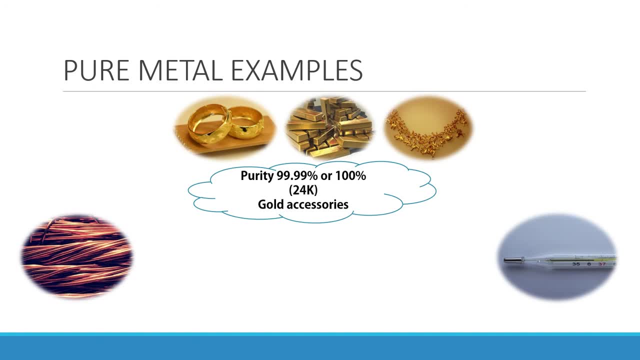 of gold are made of 100% pure gold, with no other metals mixed in it. Pure copper, which are very well known for their excellent electricity and heat conductivity, are widely used in electrical wiring works. Mercury is the only pure metal which exists as liquids at standard condition. 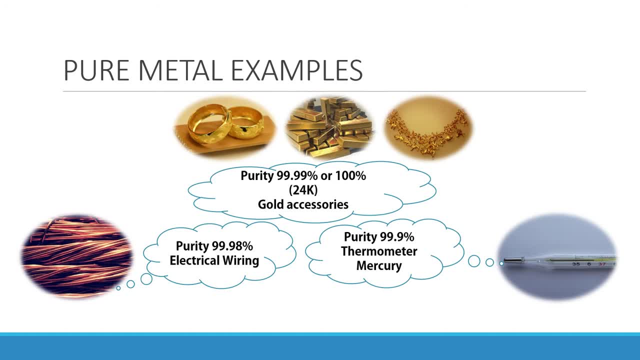 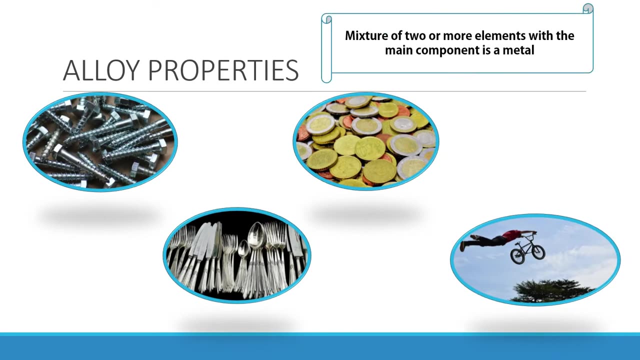 of temperature and pressure. Pure mercury liquid is often used in laboratory thermometers and shows high accuracy in temperature readings. Next, let's have a look at alloys and their properties. Alloys are made of mixtures of two or more elements, with metal as the main component. Alloys are more durable as compared. 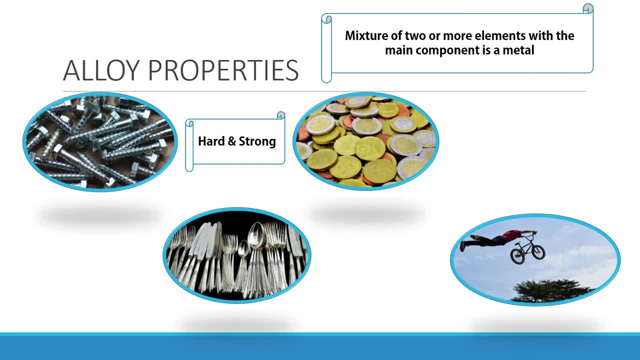 to pure metals. As such, alloys are harder and stronger. Alloys resist corrosion better than pure metals. This is because alloys are added along with mixtures of elements such as chromium or copper. As such, they form a stable, passive film upon reacting with water and oxygen. This is the reason we don't see rusted coins, as they are made of alloys. Besides that, metals made of alloys are shinier and gives it a more appealing aesthetic value. Some alloys are low density. They are made to become 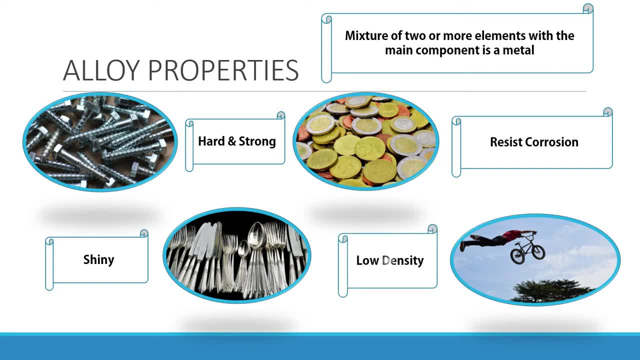 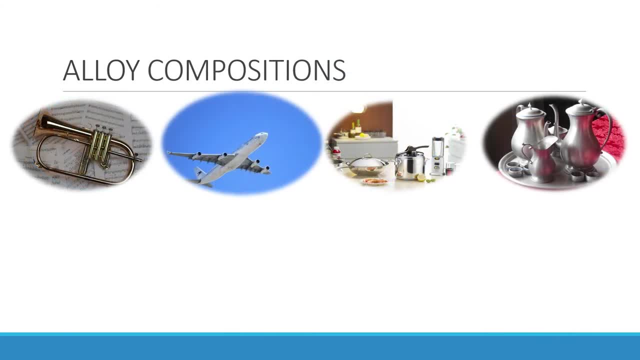 light-weighted. For instance, many bicycles are made of light-weighted alloys to reduce users' endurances. There are many things in our lives that are made of alloys. For instance, airplanes are made of light-weight duralumin, which is composed of 93% aluminium, 3% copper, 3% magnesium and. 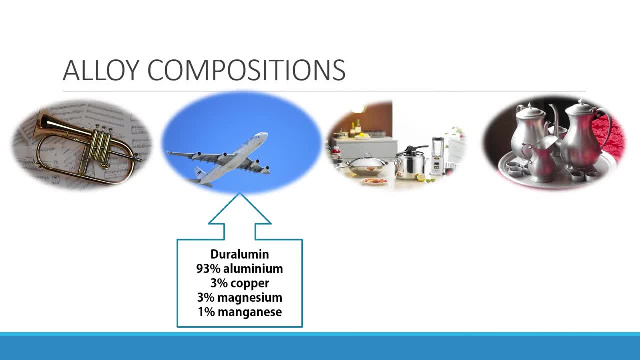 1% manganese- Our daily life consumption depends on kitchen appliances and utensils, such as windows- were made of stainless steel, which was made of 74% iron, 18% chromium and 8% carbon. Apart from this, pewter products are also made of alloys made of 96% tin, 3% copper and. 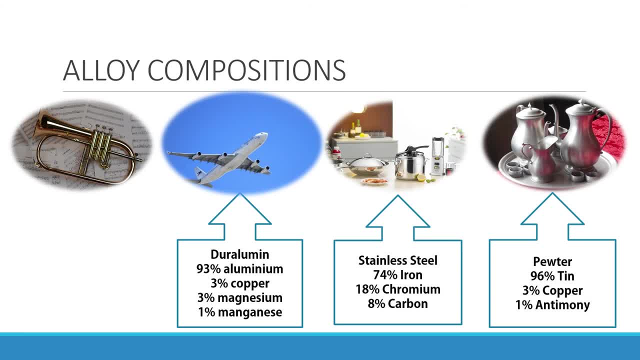 1% antimony. Most musical instruments are also made of alloys. For example, the brass trumpet is made of 70% copper and 30% zinc. 23.4 Alloys can also be made of brass trumpets: 40.1. 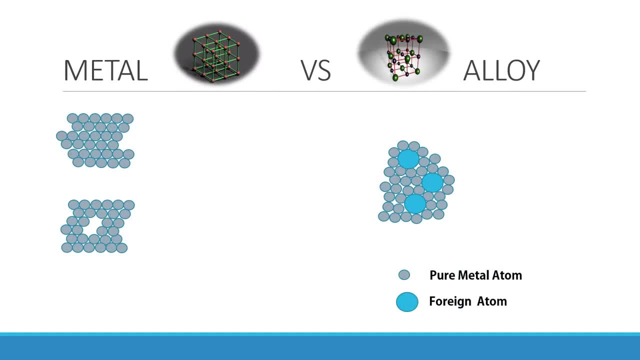 5.2, 5.1.. Moving on, let's try to understand the reason why alloys are harder and stronger compared to pure metal elements. Well, when external forces such as hammerings are applied on pure metal, the pure metal atoms can easily slide over one another and occupy the empty spaces available. 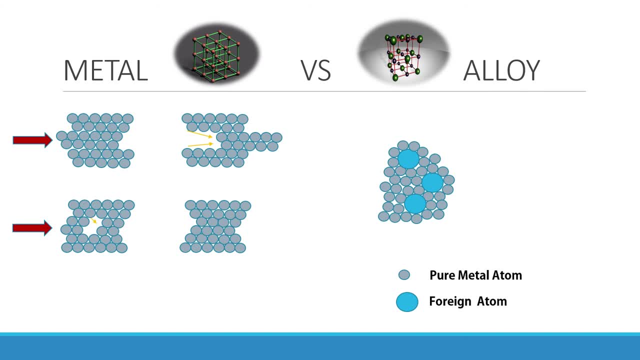 Hence the pure metal will also have a different shape when hammered, as the pure metal atoms fill in the empty spaces and form new structure. However, in alloy, the presence of foreign atoms along with the metal atom prevents the metal atom from sliding over one another, especially when the foreign atom size is different from 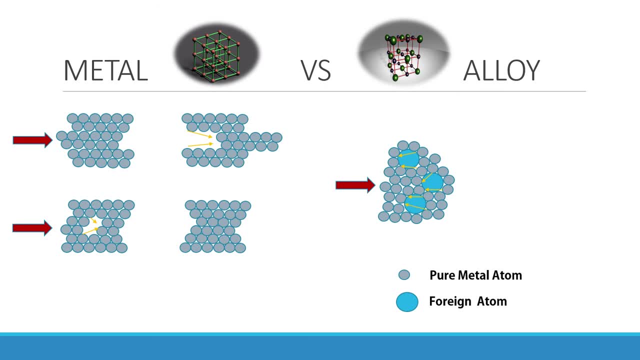 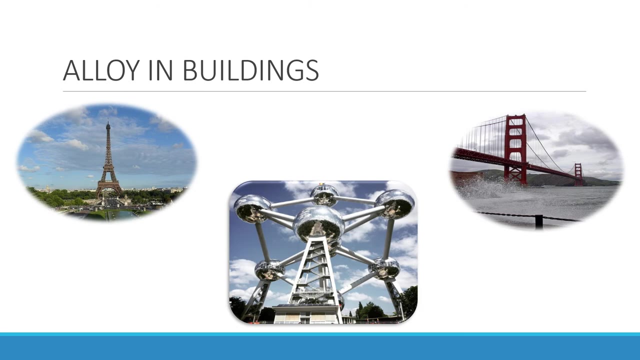 the main metal atom. As such, the alloy stays in its original structure when forces are applied on it. So some of the iconic buildings in world history are also made mainly using alloys. In 1889, the Eiffel Tower of Paris was built using wrought iron with low carbon content. 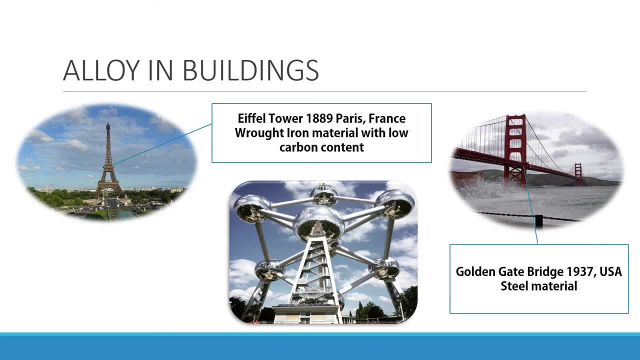 Meanwhile, in 1937,, the Golden Gate Bridge in United States America was built using steel. In 1958,, the Atomium was built using stainless steel material in Brussels, Belgium. The Atomium was also used in the construction of the Eiffel Tower of Paris. 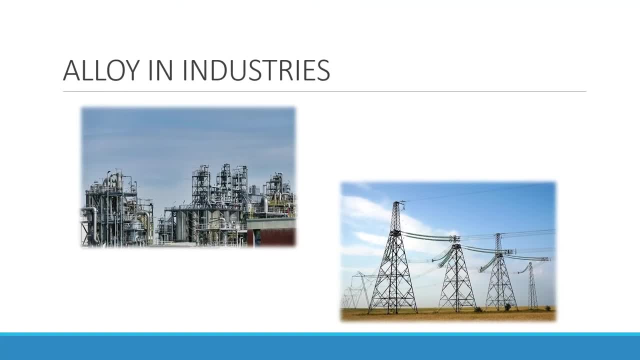 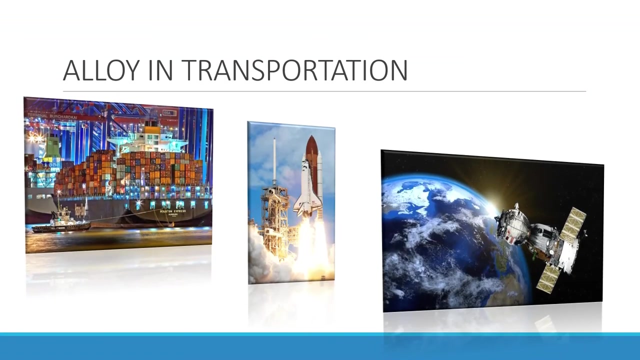 Alloys are fundamental in building oil refinery plants and they are widely used in manufacturing industry as machines, piping material, electrical wiring materials. Not to forget, we use electricity which is transferred by power lines which are made of alloys. In fact, our daily life transportations are made of alloys. 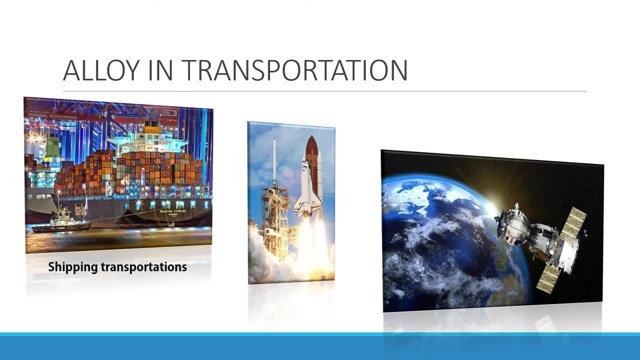